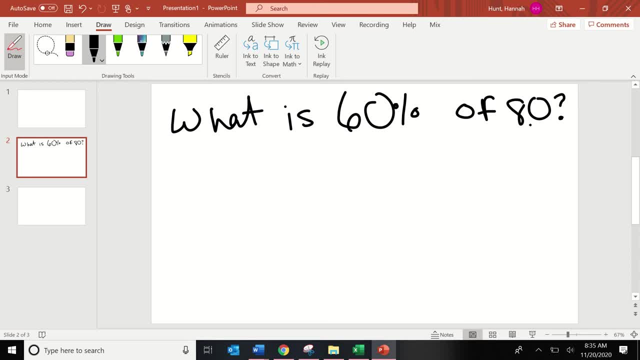 So you've probably had this exact situation- maybe not with these numbers, but you've probably had this situation where it says 40% off or 60% off, And you say, well, what's 60% of 80?? Because maybe the thing you want to know is what is 60% of 80?? 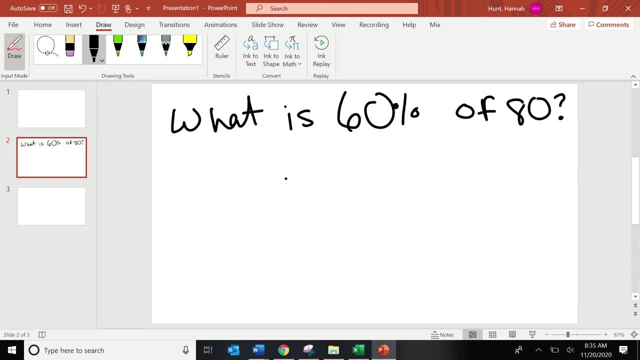 And the thing you want to buy is $80.. So the way that we're going to solve this problem, there's actually a couple different ways to solve it. There's a short way and a long way, And the state wants you to learn the long way. 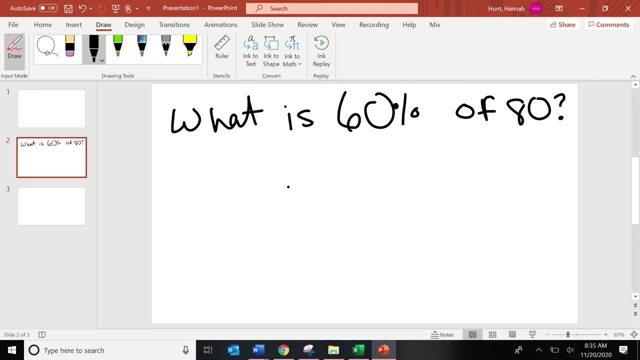 So that's what I'm going to teach you, But in the next couple years you're going to find out the short way and you're probably going to hate me, And I'm sorry, but I'm doing what the state's telling me to do. 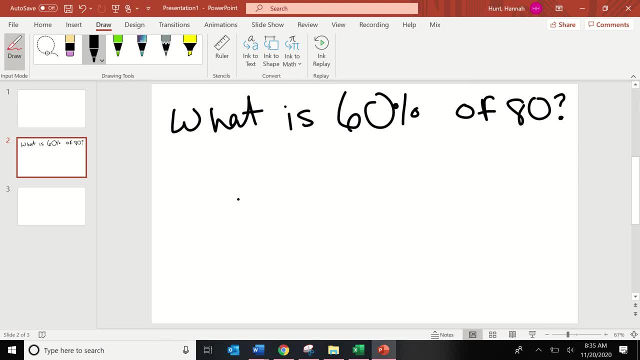 So what is 60% of 80?? Well, the way that we're always going to start is we're going to set up part Over total. This is a proportion. Part over total equals percent over 100. And in the video he says whole instead of total. 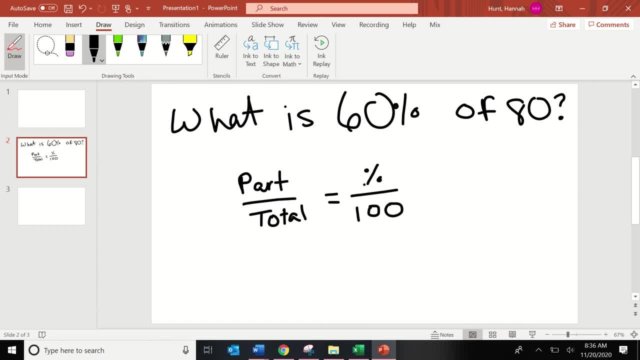 I don't know. I just like the word total better. So part over total equals percent over 100. And when we have a problem like this, what is 60% of 80?? The part would go here. The percent is obviously here where there's a percent sign. 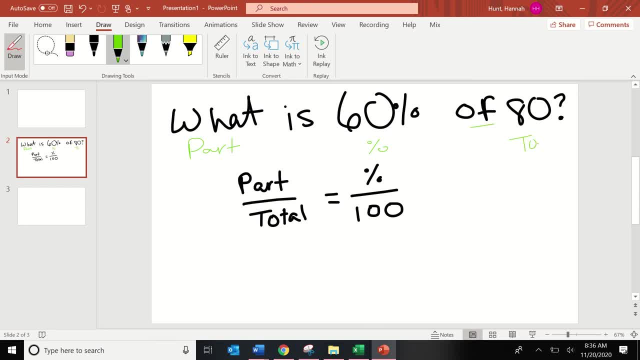 And then we're going to set up the whole- And the total is here after the word of- So for this problem, what we want to do is just take the numbers we know and put them into this proportion And then solve for the part, which is what we're missing. 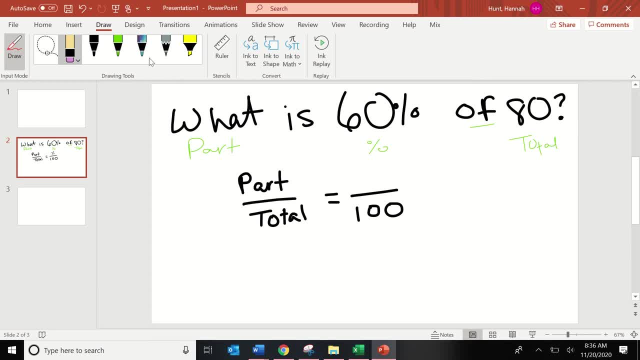 So we know what the percent is, So we're going to- right here, we're going to put a 60.. We know what the total is, So right here, we're going to put an 80.. So, basically, we were saying: 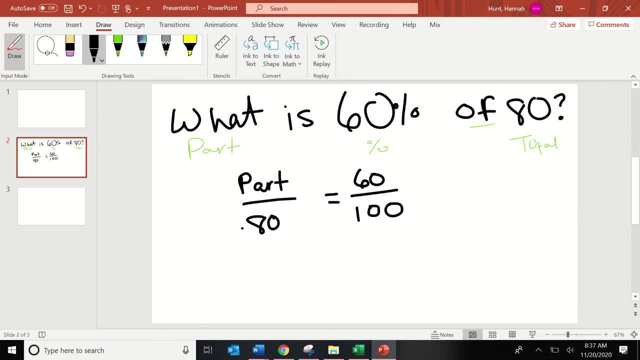 What fraction out of 80 is the same as 60 out of 100?? And we can't really go when it comes to solving proportions. We know how to do that. If there's something I can multiply here to make it easy, I would do that. 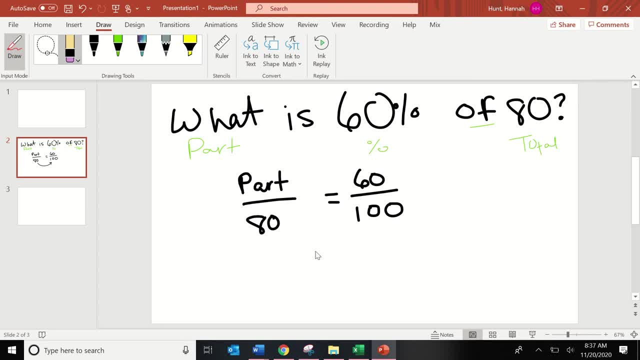 But 80 times what equals 100? That's not really going to work. So I'm going to cross, multiply and divide. So then I have 60 times 80, is what 4,800.. Yes, 4,800. 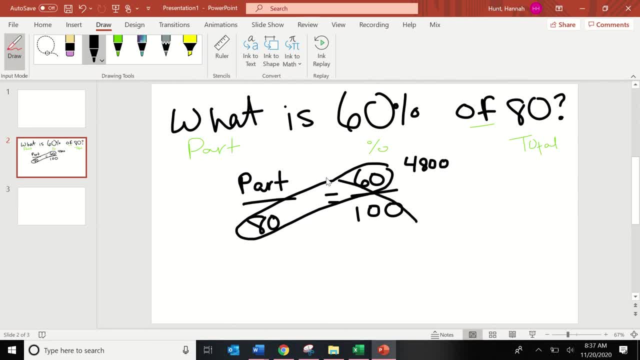 And I would divide it then by 100. Because I know that the number I'm missing times 100 has to also equal 4,800.. So 4,800 divided by 100 is 48.. So what is 60% of 80?? 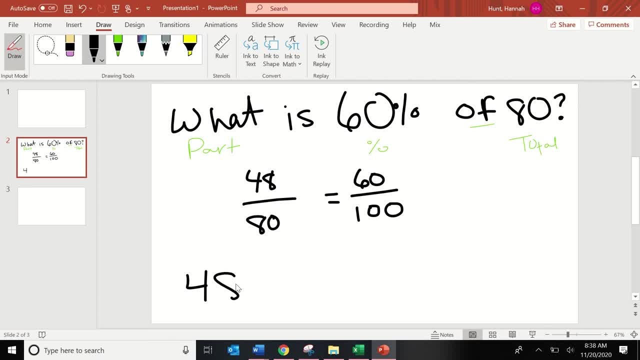 48 is 60%. 60% of 80. 80. So what that means in real life is if I'm buying an $80 jacket for 60% off, then I can take off $48 from the price. Okay. 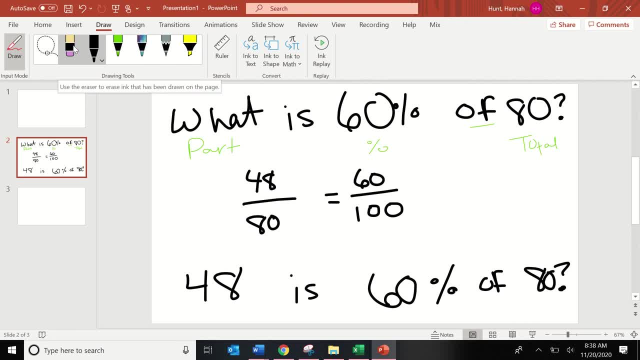 I'll do one more and then hopefully you'll be able to go ahead and do those IXLs. So let's say, Oh, I didn't need to erase that, Let's do that. Let's say, what is? Ooh, this time I'm going to use a number that's bigger than 100,. 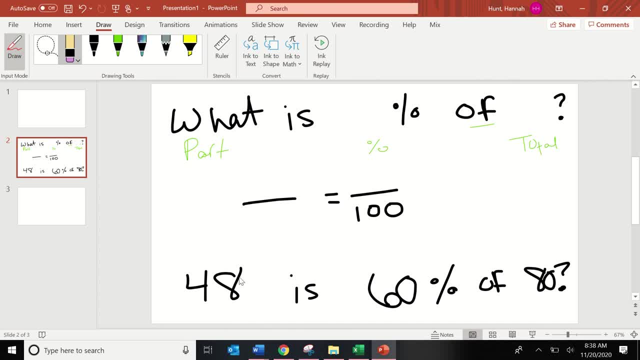 because that always confuses everyone. So in case you get a problem like that, you'll know what to do. So this one will say: what is 120% of 45?? Okay, So here's where people get confused. It'll be a question like: what's 120% of 45?? 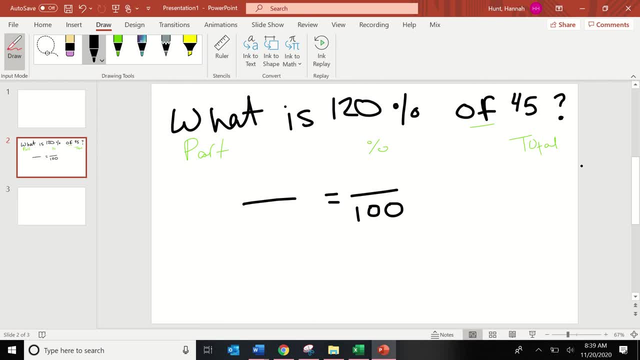 And you'll be like 120%. what is that? But it's not really that hard. You've heard people say something like: I'm going to give 110% of my effort. Well, what does that mean? It means I'm going to give all of my effort and then some. 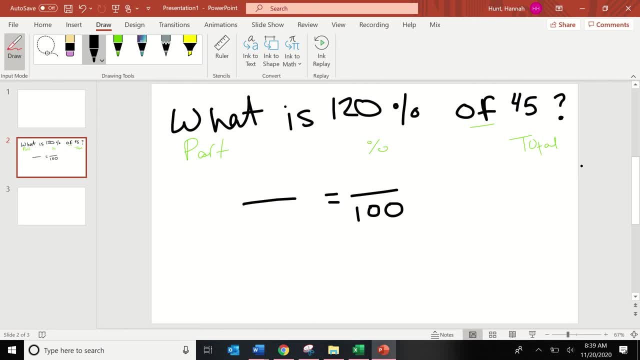 So if I have like, for example, if I go shopping and I spend 120% of the money I bought with me, well I'm in debt because I spent more than what I had. So 120% means more than all of it. basically. 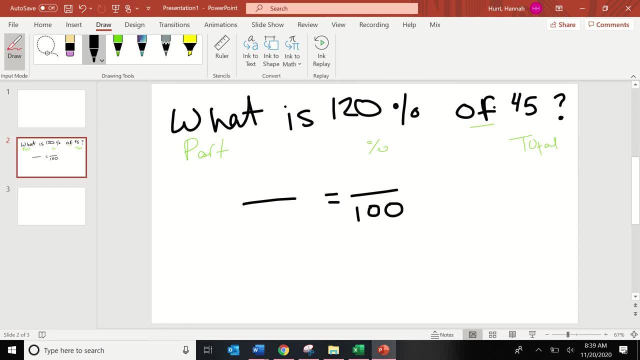 So what is 120% of 45?? It's actually more than 45.. Okay, So what is 120% of 45?? It's actually more than 45. But the way, The way that we solve it with this proportion, is the exact same way. 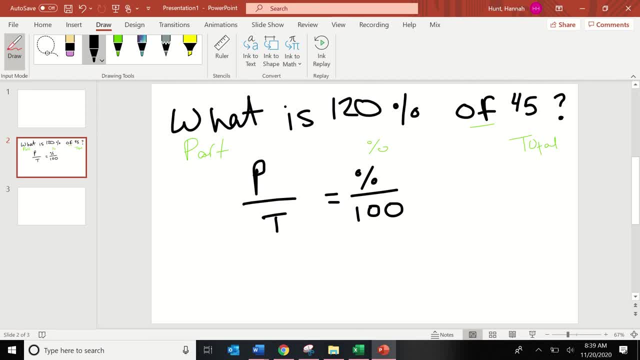 So we have: part over total equals percent over 100.. I would say, okay, the part is what I'm missing. So I need to find out what goes here. I know the percent is 20.. Nope, not 20, 120..